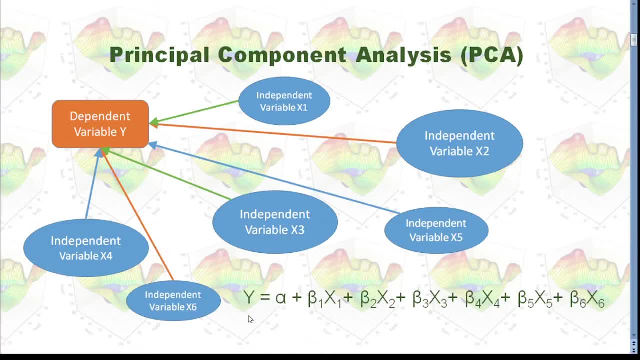 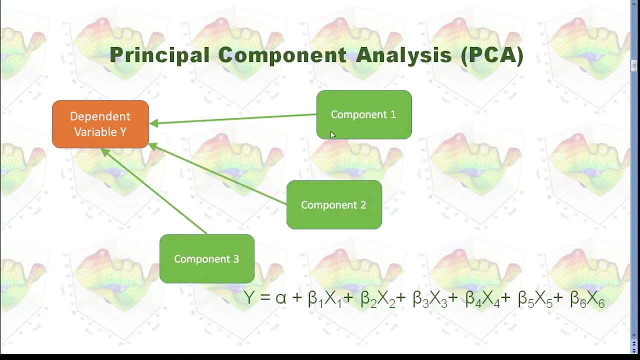 and then we can build our model based on this formula. If we want reduce dimensionality, we can build principle component like component 1, component 2, and component 3.. And then we can convert our original model to this model, which this one is: component 1, component b and component 3.. 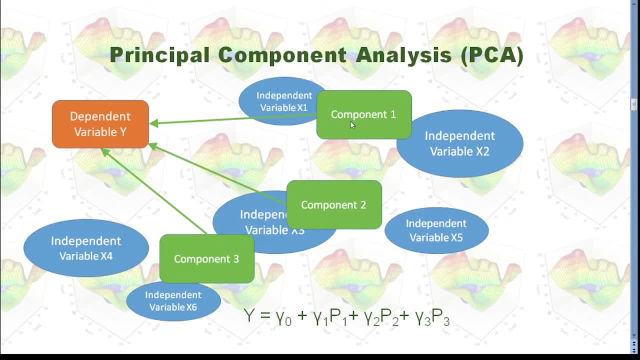 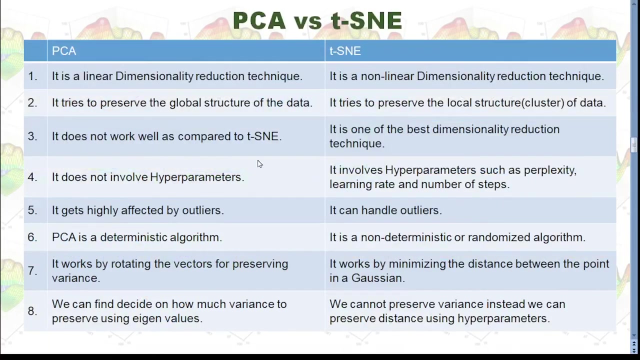 Please remember all those: principle component is linear combination of all the independent variables. But it must be a linear combination. This is limitation of principle component analysis. Now let's compare PCA and t-SNE. Like I just mentioned, PCA is a linear dimensionality reduction technique. 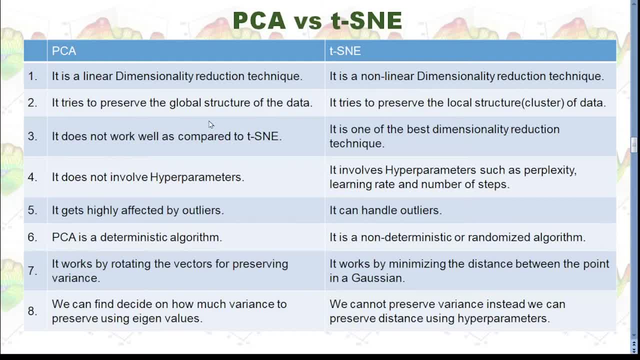 and t-SNE is nonlinear technique. Then PCA tries to preserve the global structure of the data. t-SNE tries to preserve the local structure or the cluster of the data, And PCA does not work well as compared to t-SNE, And t-SNE is one of the best dimensionality reduction technique. 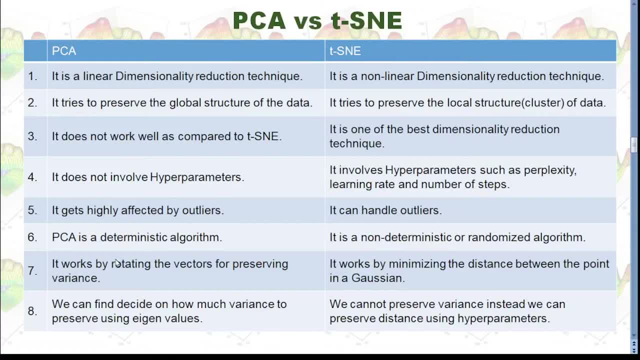 PCA does not involve hyper-parameters, While t-SNE involves hyper-parameters such as perplexity, learning rate and number of steps. We are going to check all those hyper-parameters in detail later And PCA gets highly affected by t-SNE. 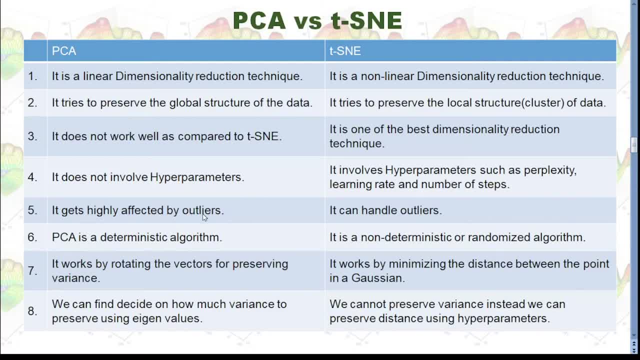 Highly affected by outliers. While t-SNE can handle outliers, PCA is deterministic algorithm, While t-SNE is a non-deterministic or randomized algorithm. PCA works by rotating the vectors for preserving variance, While t-SNE works by minimizing the distance between the point in a Gaussian. 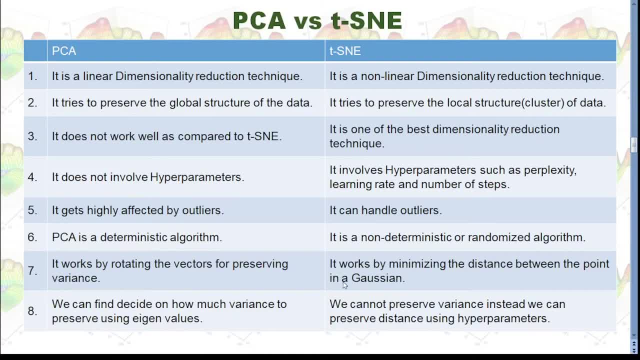 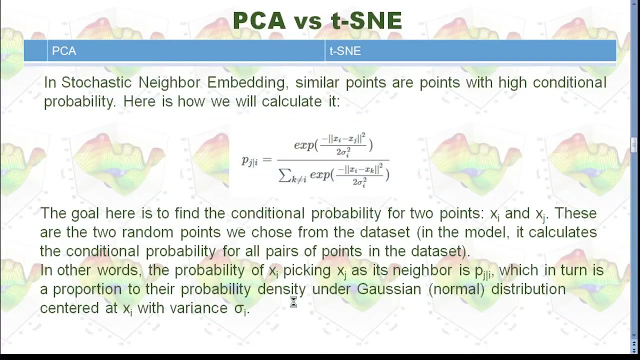 I'm going to explain that in detail later. In PCA we can find and decide on how much variance to preserve using eigenvalues In t-SNE. we cannot preserve variance. Instead, we can preserve distance using hyper-parameters In t-SNE. 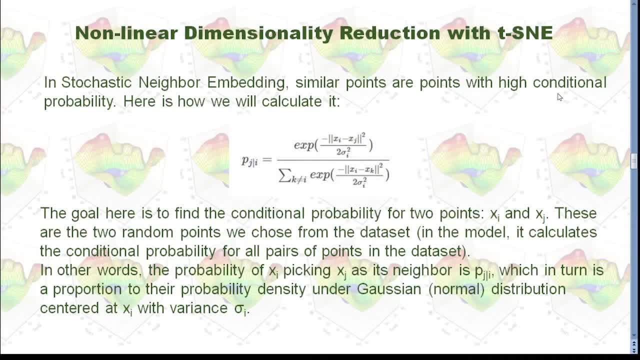 similar points are points with high conditional probability. We use this formula to calculate conditional probability. Here we have two points, xi and xj, And this part means the distance between xi and xj, And this is the variance which is centered at xi under normal distribution. 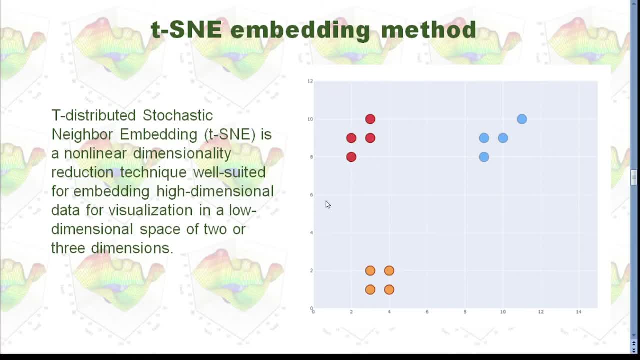 Let's take a look at this example. The goal is to reduce this two-dimensional data to one-dimensional data. We have data points here and also here. Please remember, when we train our model, we don't have any label for those data points. 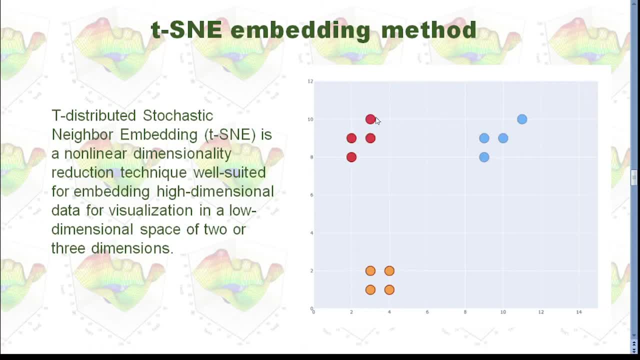 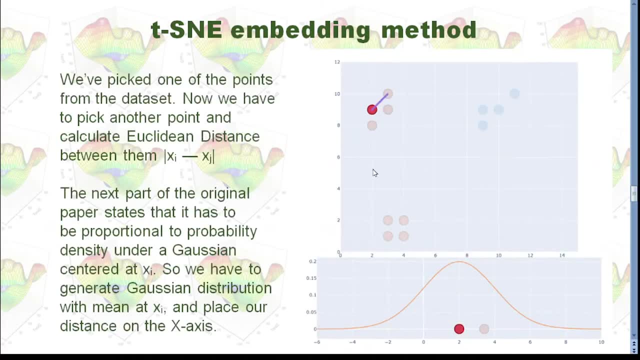 Just imagine when we train the data. there is no color for those data points, They are all gray. And then we pick up one point, Let's call it xi, And we are going to measure the distance between this xi and another point. 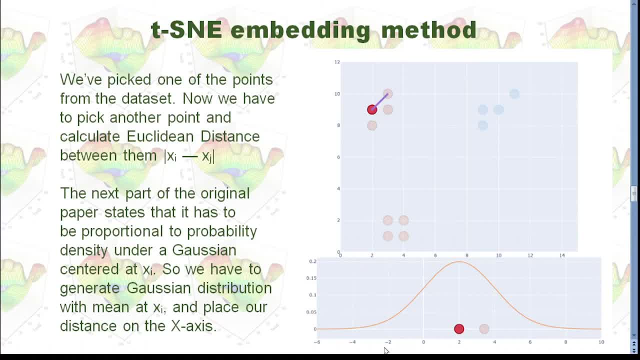 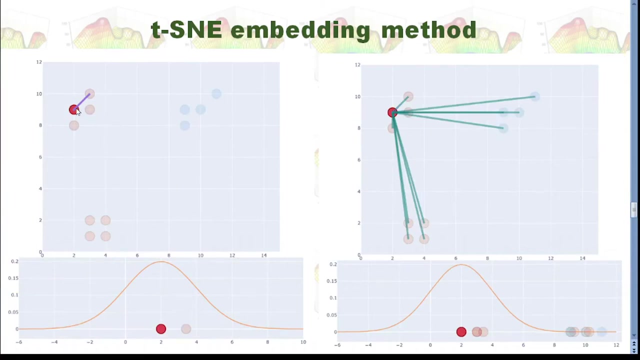 At this time we are going to use normal distribution Because xi is this data point. it will sit in the middle of the distribution And another data point will sit here. So this is the graph I just showed you And, similarly, 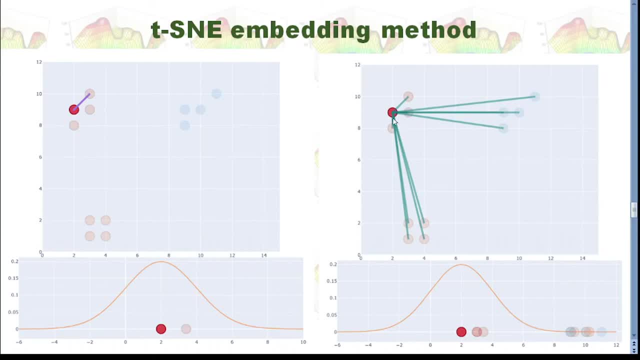 we are going to measure the distance between xi and all other data points, And then you can draw the graph like this, Because this is the first data point, First one, And then the second one here, And then all the other data points. 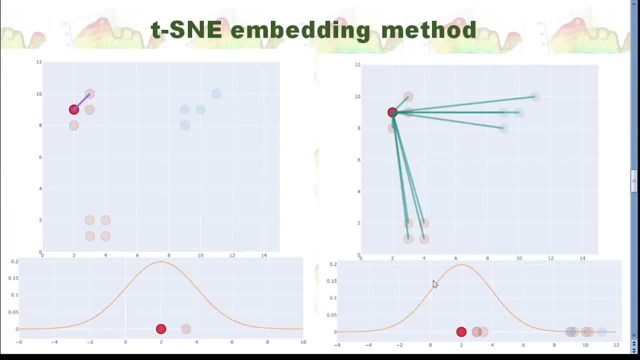 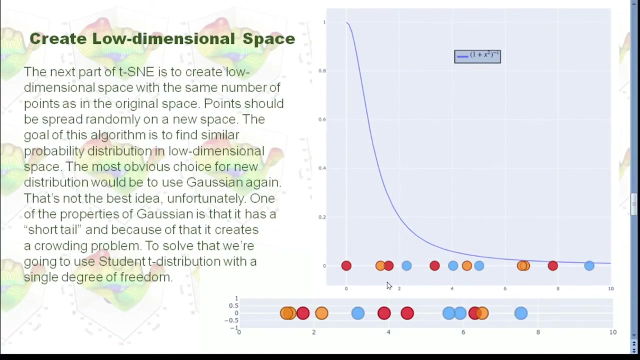 Please remember, in this process we are using normal distribution. After we calculated all the distances among all those data points, we want to reduce this two-dimensional data to one-dimensional data. Now we are going to put all the data points into low-dimensional space. 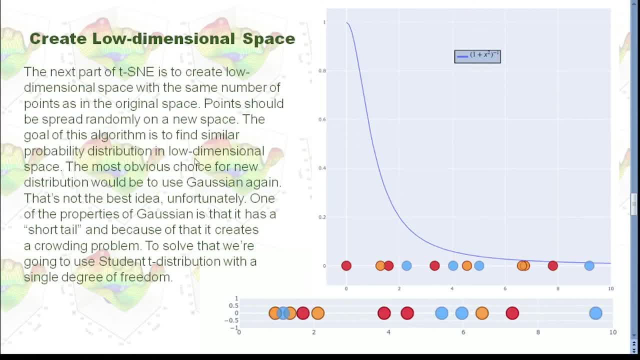 In this case, we put into one-dimensional space And now, if we still use normal distribution and it will have a short tail and because of that it creates a crowding problem, To solve that we are going to use student t-distribution. 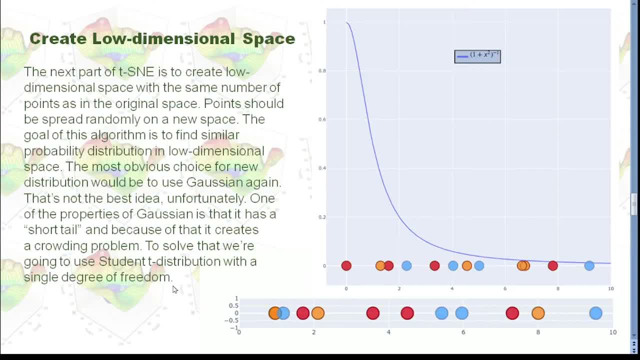 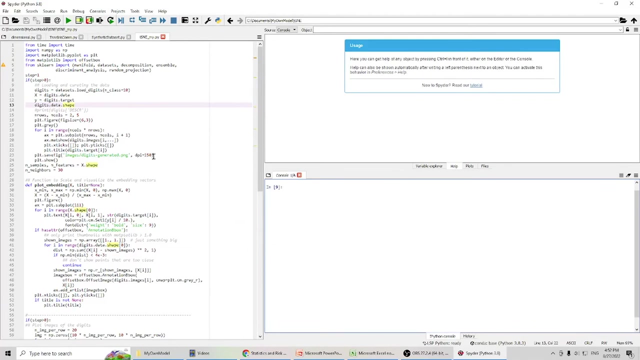 with a single degree of freedom. That's why we call this method t-SNE. The t stands for student t-distribution. Now let's go to Python to see how can we implement that. In this video I'm going to use 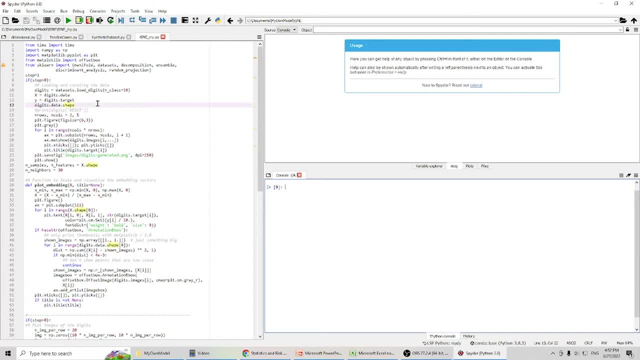 some digit images for our data analysis. I'm going to use those digit images for the data analysis from 0 to 9.. One image is composed with 8 times 8 digits, So this is 64-dimensional digits data set And then 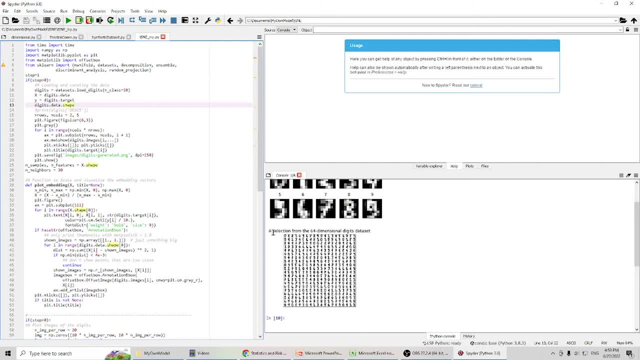 I generated this 20 times 20 digit map, So one number is one data point for me. Now I'm going to classify all those data points with PCA method and t-SNE method. Now I'm computing PCA projection. You can see: 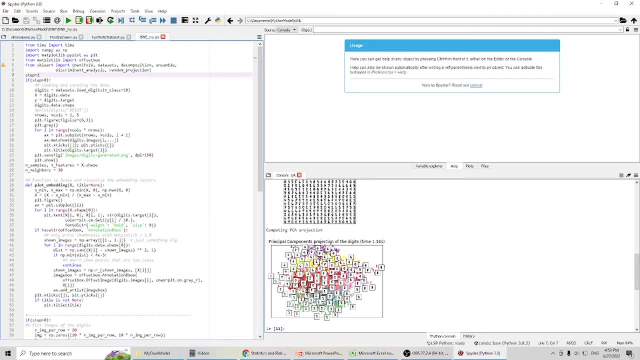 this is the result of the PCA projection. You can see I have 4 here and 6 here, But a lot will overlap here And I spent 1.16 seconds for this PCA projection, So we reduced the dimension from. 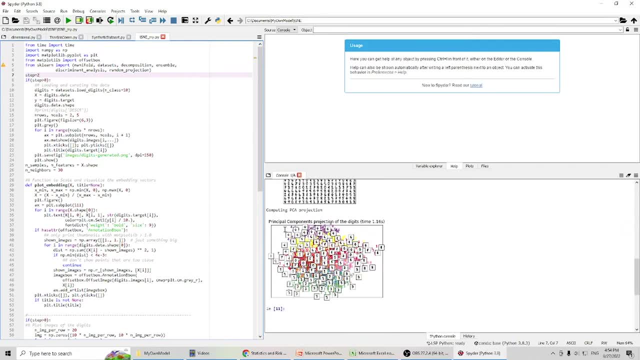 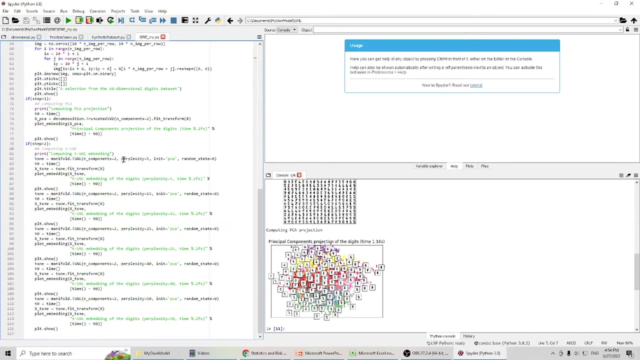 64 to 2-dimension. And please remember, in this data set you can see I pull the data, put into x array And then when I do the PCA method, here I only used x. The x PCA is here. 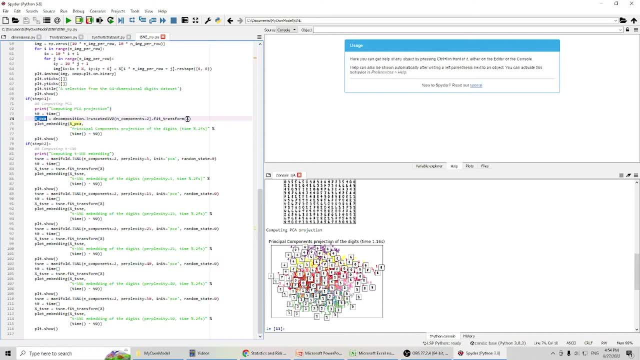 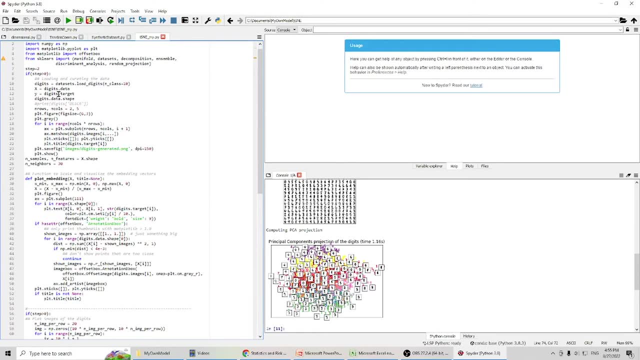 It's defined here. You see, I only used x And I didn't use digits dot target. The digits dot target will tell us this number is 0 or 1 or 2 or 3.. So we can see that. 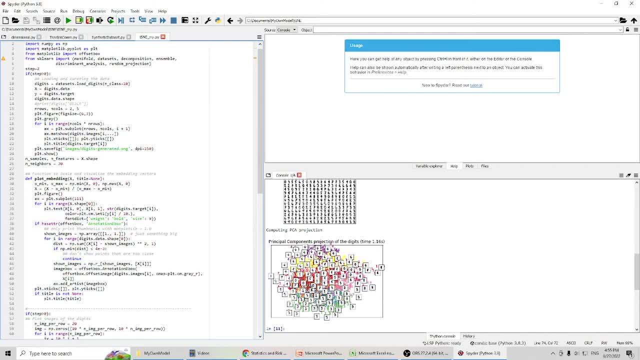 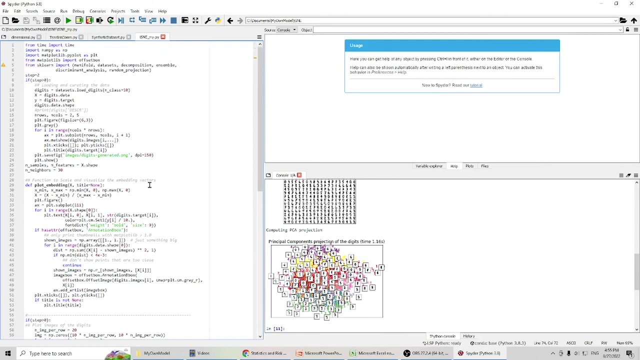 we can see that we can see all those labels here. But when we use PCA projection we didn't use all those labels. So the PCA method here is unsupervised machine learning And similarly we can do PCA projection test again. 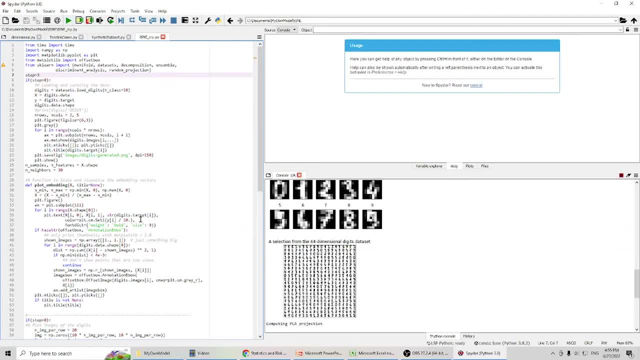 And when we use the PCA projection test again, we will do the PCA projection test again. It's done. And then it started the t-th knee First step. I used as the perplexity and it took. it's hard to see. okay, let it finish the second. 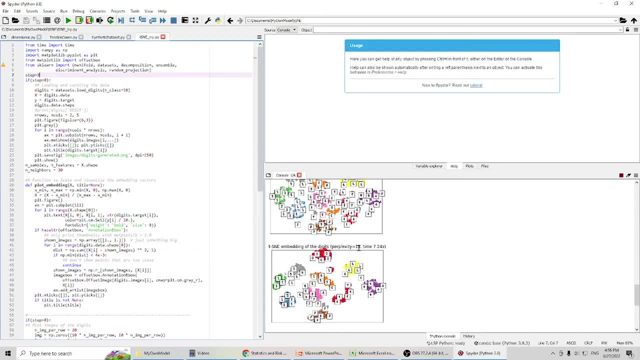 step, I use perplexity equal 15 and then I use perplexity equal to 25. this is about the tuning of the model and we can choose all those parameters, hyper parameters to to our model, and in Python the perplexity is from 5 to 50, so okay. 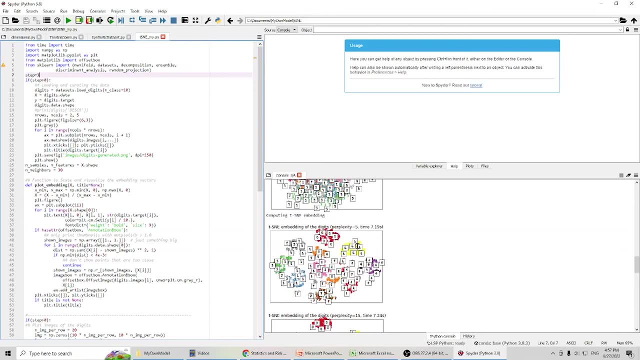 now we can go back when we use five as our perplexity. you see, the data still have a lot of overlap and it took 7.19 seconds and if I use perplexity 15, it took 7.24 seconds. so you can see it. 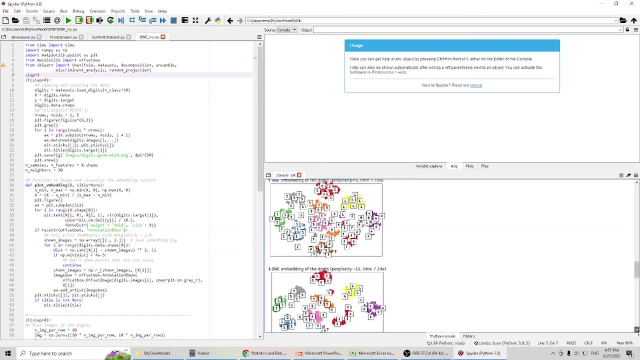 will take longer time, but we will get better result. you can see all those clusters. they are separated, and if I use perplexity 25 it will take even longer- 8.44 seconds- and the result is kind of similar with when we use perplexity equal to 15. so this is kind of balance. if you use 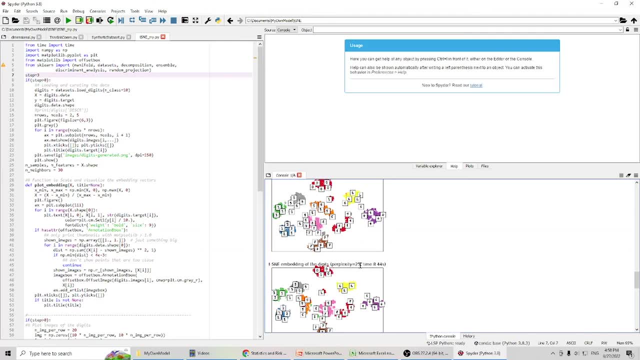 larger number of perplexity, of course you can get better result, but it will take longer time and it needs much more computer power. and this is only a very simple example. when you do the real like machine learning for real project you might have like millions of data and if you have a large number of perplexity of 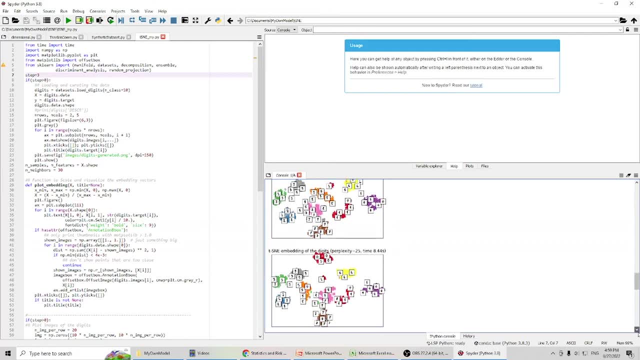 course it will take much longer time. and you can see, even we take perplexity equal to 40 or 50, the results remain almost the same. so in this example, maybe we can stop with perplexity equal to 15. I will upload this Python program, the source code, to my github so you can. 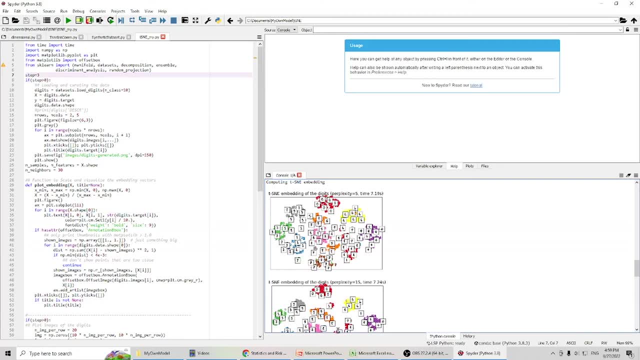 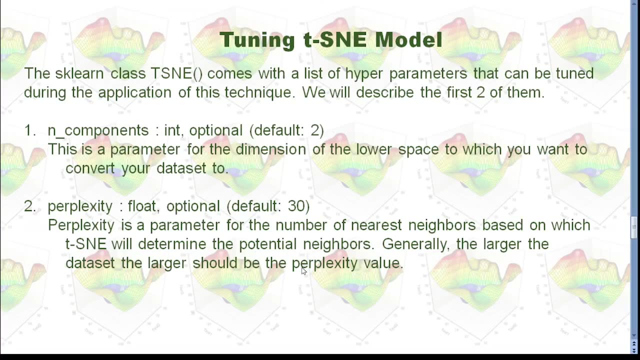 download the source code and try it out and see if it works or not. I will upload this Python program, the source code, to my github so you can download the source code and try it out and see if it works or not by yourself. when we use Python for our t-thne model, there are several hyper parameters. you 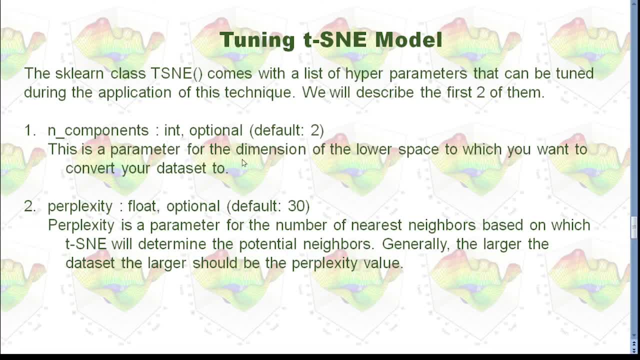 can tune for your model. the most important two are: the first one, the n components. that means the dimension of the lower space, and in this case we will use two because we want reduce our dimensionality to two-dimensional space. and another one is perplexity. the default is 30. you can try the different.